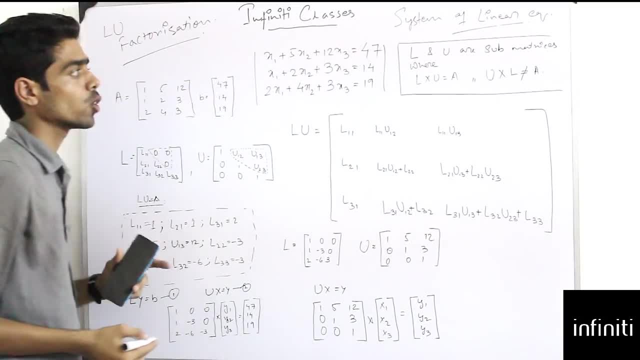 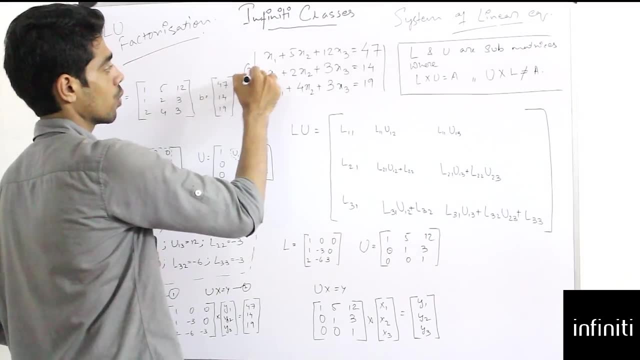 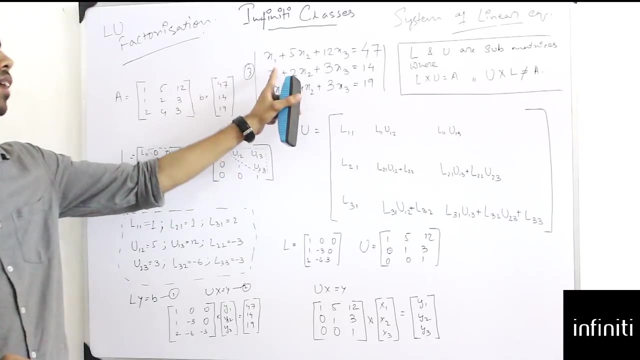 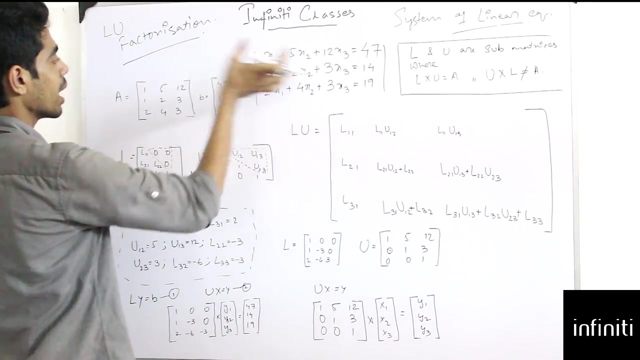 three unknown quantities- x1, x2 and x3- and to find these three unknown quantities we require a minimum of three equations. okay, so we have one, two and three equations over here. okay, so by these three equations and by using LU factorization, we will calculate the values of x1, x2 and x3. okay, so this is my equation. okay, I'll converting my equation into: 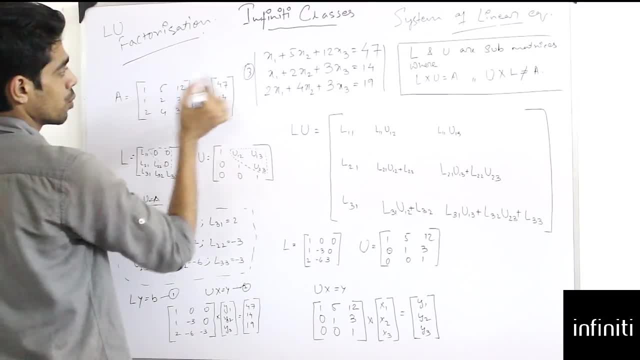 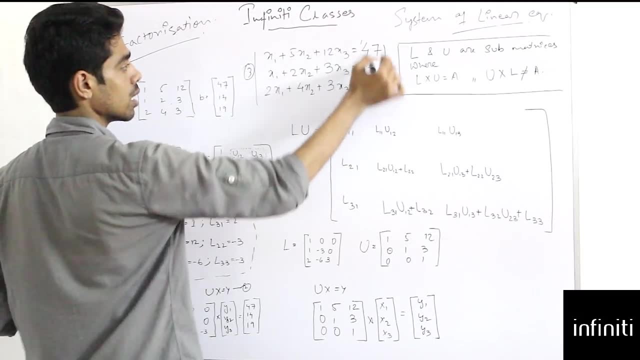 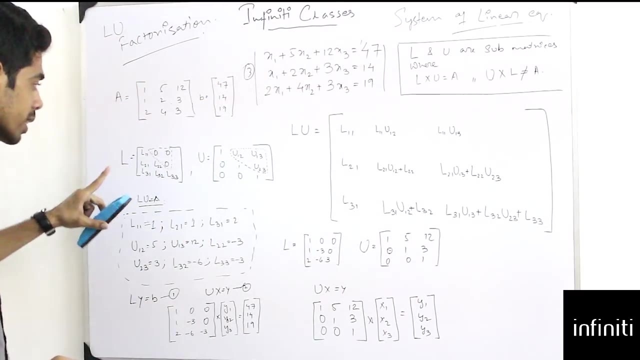 something like this: matrix: 1, 5, 12. 1, 5 12. 1, 2, 3, 1, 2, 3, 2, 4, 3, 2, 4, 3. okay, and this is my b. okay, this all is my a capital a and this is my small b. this is my small b, okay. so what is l? and u? lu are two. 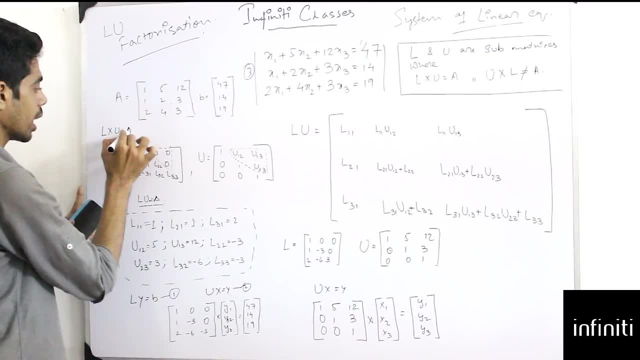 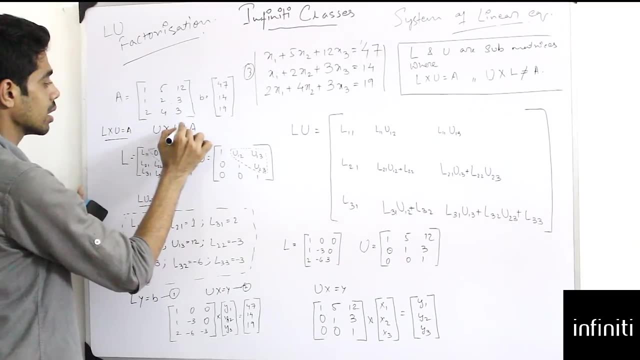 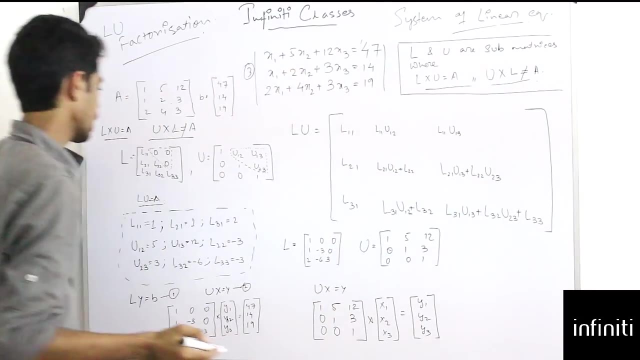 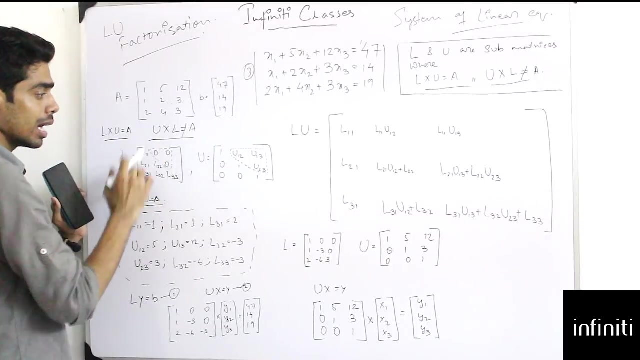 which is: l cross u is equals to a. that doesn't mean u cross a. u cross l is equal to a. that doesn't mean that. okay, l cross u is equals to a. you have to follow this. okay, now we have l. we have u. okay, what is l? l? 1, 1, 0, 0. okay, in l we have upper triangle 0 and in u we have upper triangle as u. 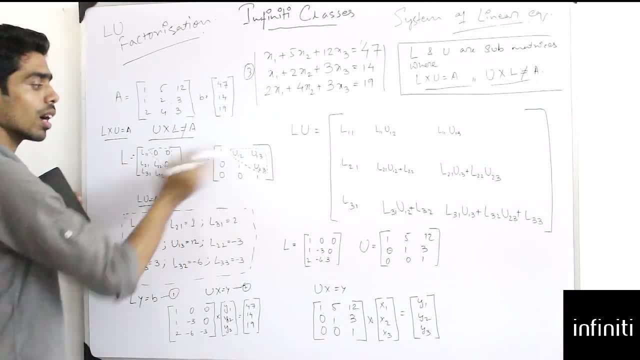 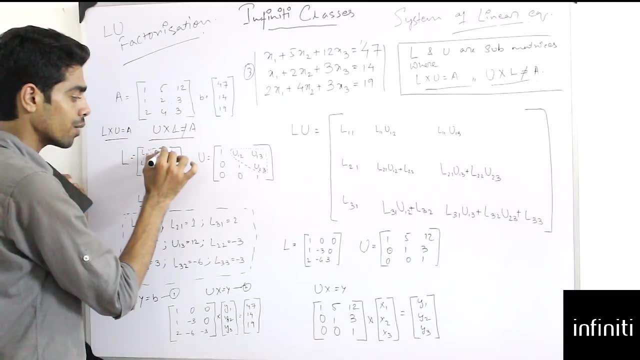 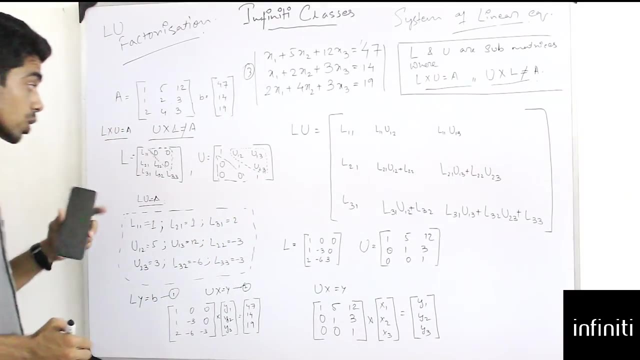 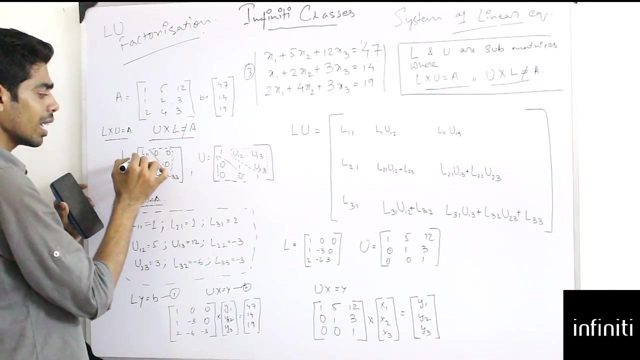 and everything diagonal is 1 and everything opposite to that diagonal is 0. or you can remember like that: in l, the upper triangle is a 0 and u, the lower triangle is a 0. okay, so for l, the upper triangle is 0 and for u, the lower triangle is 0. okay, so what is l? l is l 1, 1, 0, 0, l 2, 1, l 2, 2, 0, l 3, 1, l 3, 2.. 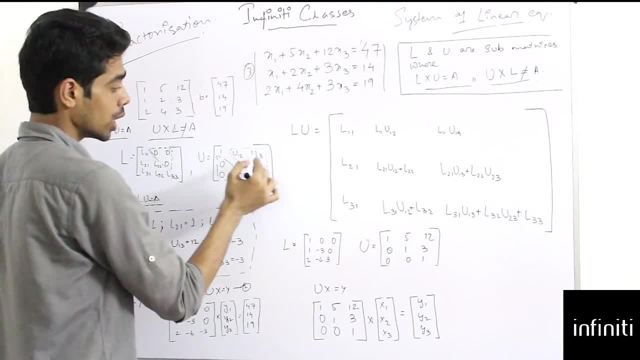 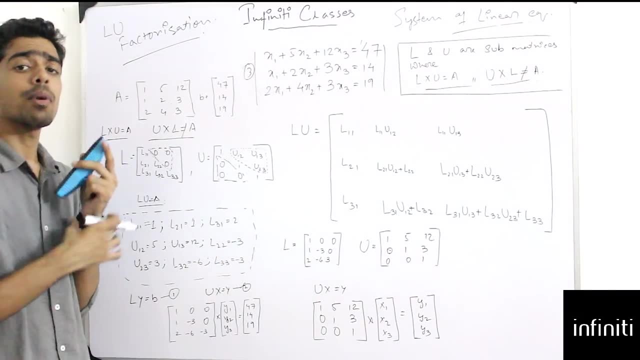 okay, and for U 1, U 1, 2. U 1 3, 0, 1. U 2, 3 0, 0, 1. okay, simple remember. for L, the upper triangle is 0 and for U, the lower triangle is 0. okay, and for U, the diagonal. 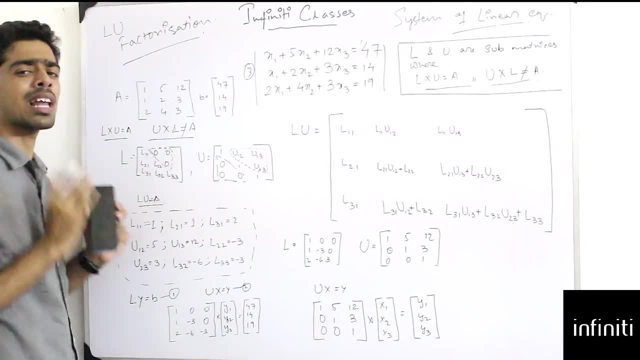 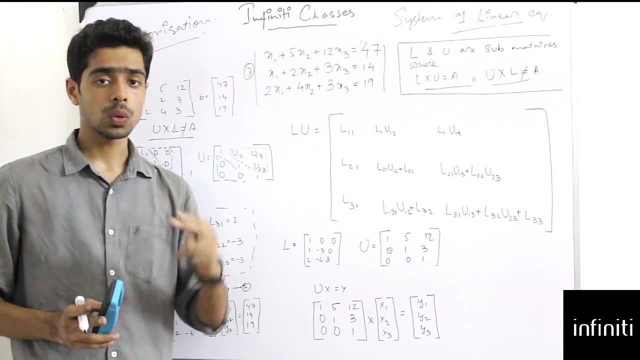 will be 1, and for L everything will be like in sequence: L 1, 1, 0 0, L 2, 1, L 2, 2, 0, L 3, 1, L 3, 2, L, 3, 3. okay, and for U you have 1, U 1, 2, U 1, 3, 0, 1, U 2, 3, 0 0. 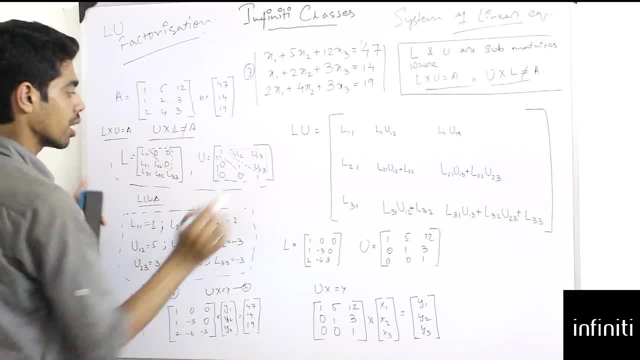 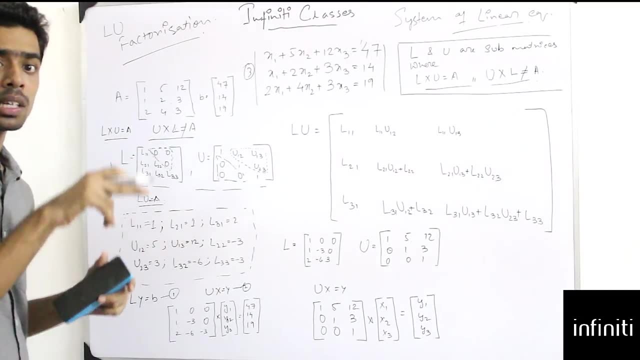 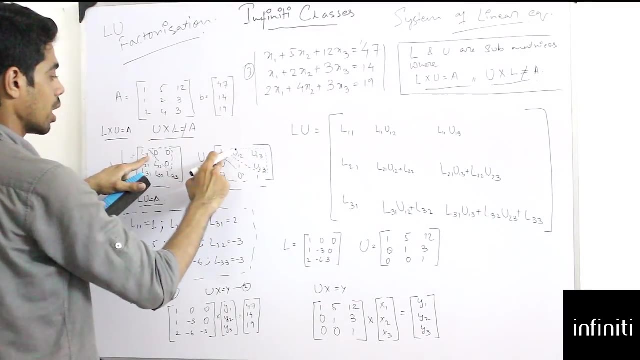 1. okay. so these two things are clear. and now, what is LU? L? U is L, cross you, like we have done a matrix multiplication, okay. similarly, L? U is 2 matrix multiplication like L 1, 1, 1 is L. now, if for matrix multiplication, 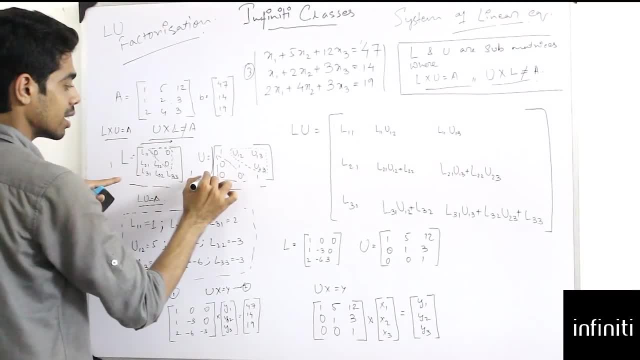 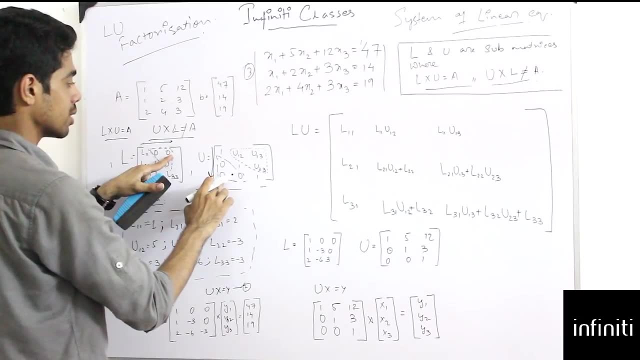 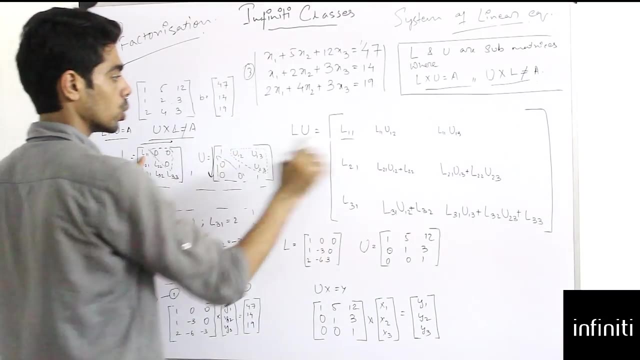 the row will be shifted like this, and for the other matrix, that column will be shifted. okay, so I'll shift 0 and shift 0. 0, 0, 0. Court 8 is 0, so my answer will be l11. now again for this: l11, u12, l11, u12. again. shift this 0 into 1 is 0. 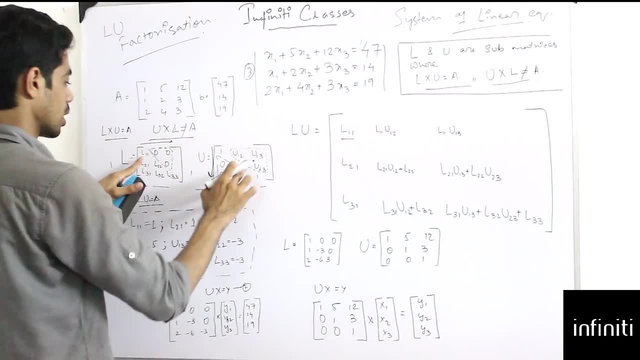 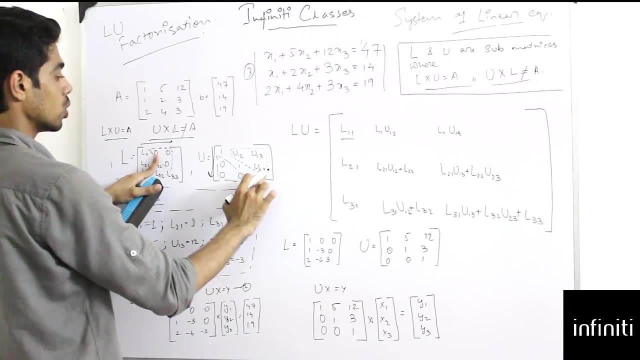 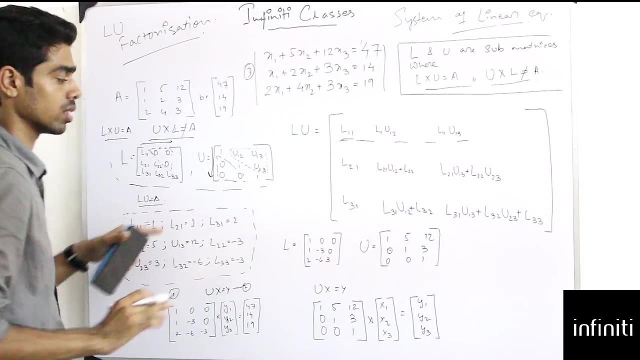 0 into 0 is 0, so nothing will be written in here. now for this. l11- u13, l11 u13: 0 into 0 to 3 is 0 and 0 into 1 is 0, so my first row operation has been completed. okay, now for the second row. 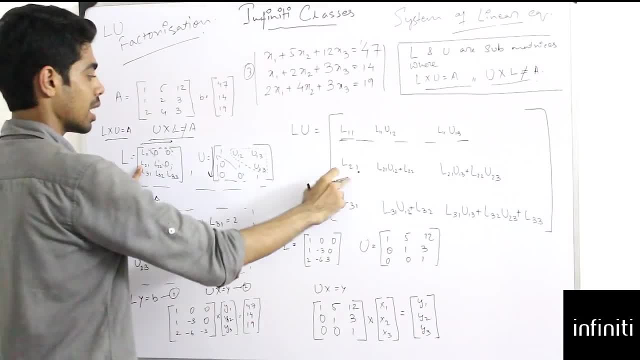 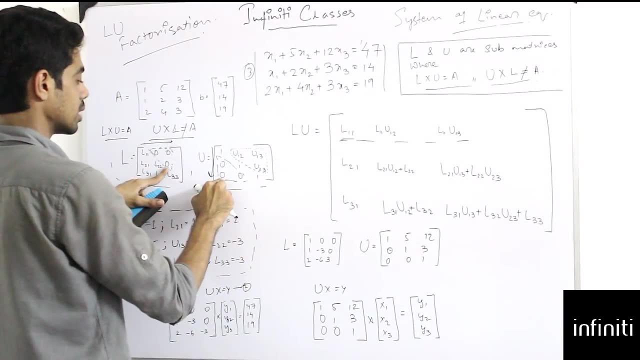 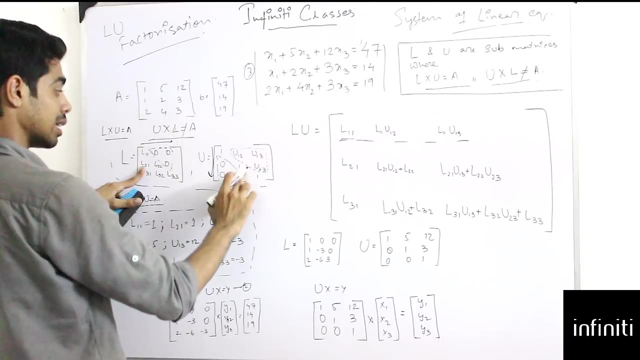 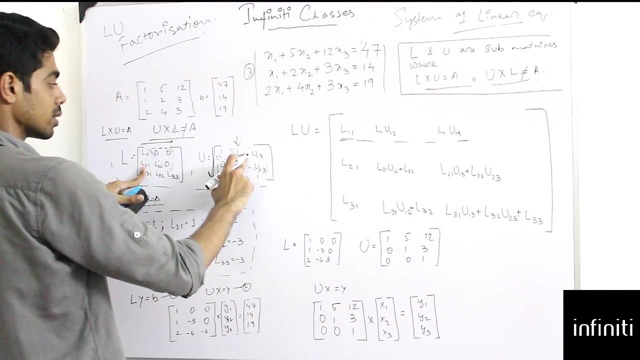 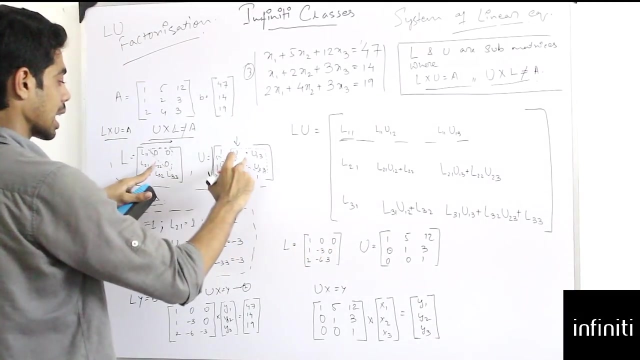 operation: l21 into 1: okay is l21. for this. l22 into 0: over here is 0 and this thing is 0, so i'll write l21. okay, now for this. again. i'll take this column: okay, now. u21. u21 is uh, u21, uh. l21 into u2, uh, u12. this will be this again. this l22 into 1 is l22. 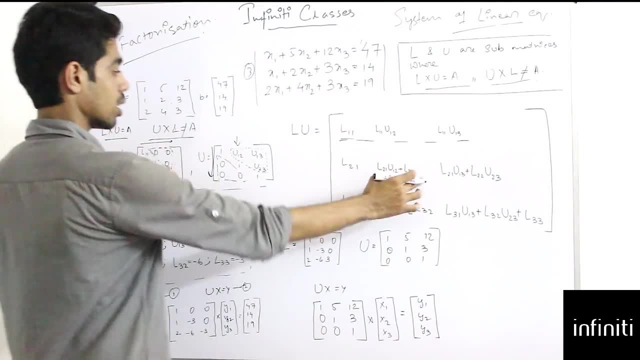 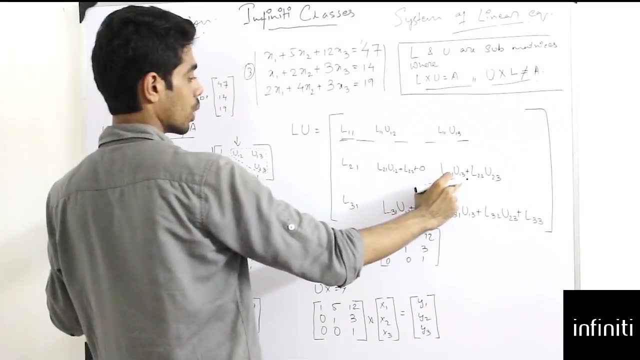 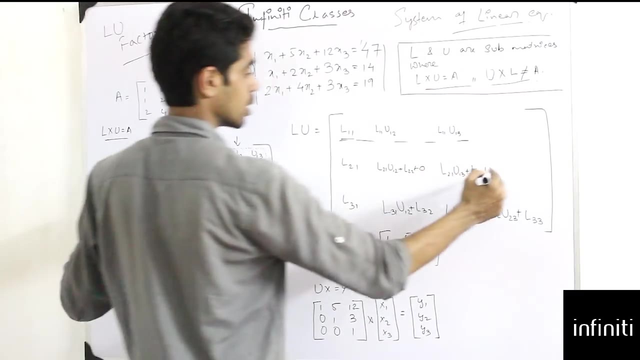 again 0 plus 0, 0 into 0 is 0, over here is 0. okay, so this will be my equation now for this: l21, u13, l21, u13, and then l22, u23, l22, u23, and then shift 0 into 1 is 0. 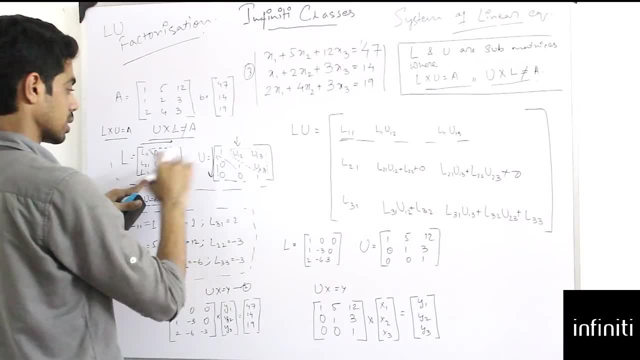 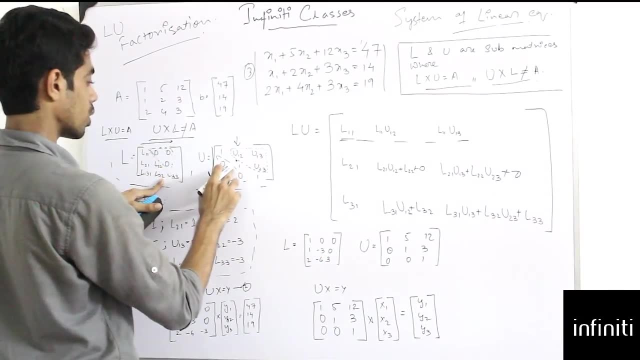 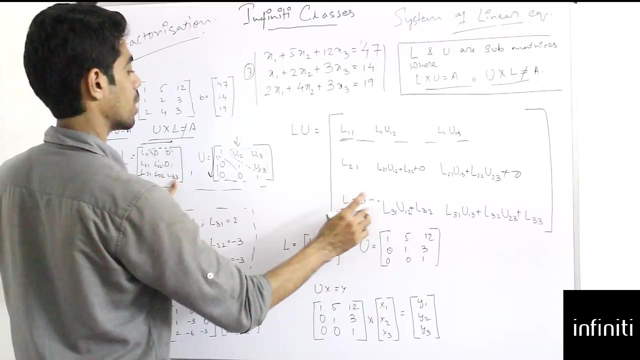 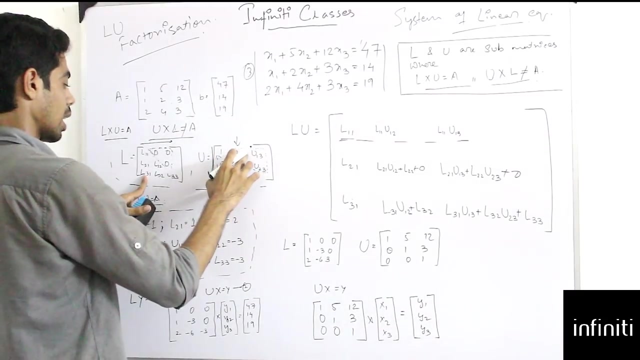 okay, now shift the same for this. okay again, l31 into 1, l31, l32 into 0 is 0 plus 0 and l33 into 0 is 0, so my last final equation will be l31. okay, now this second column: l31, u12, l31, u12- again shift. 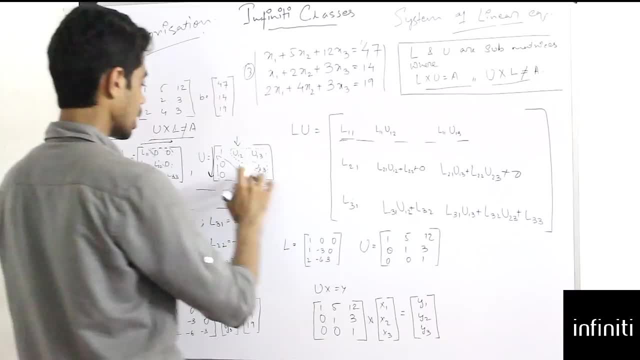 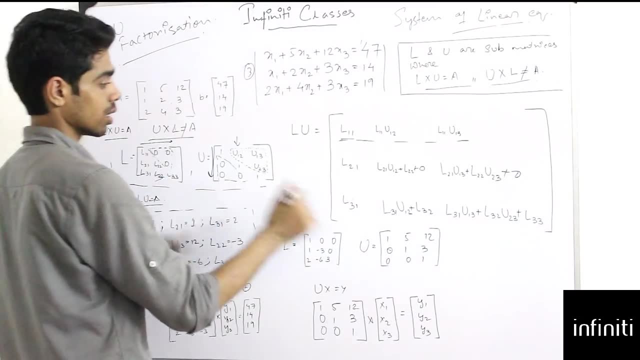 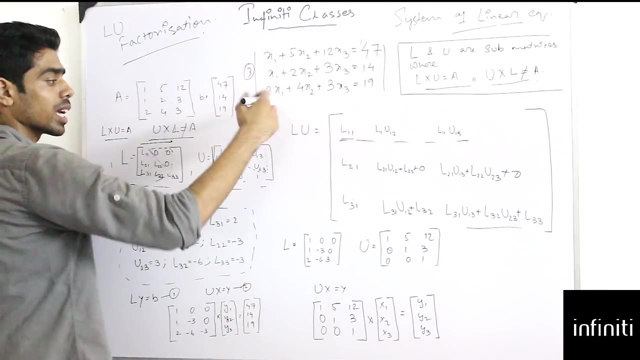 3, 2 into 1 is l32, and then shift. this will be 0. now l31, u13, l32, u23, l33. this will be my last, okay, so from this lu you will calculate lu. okay, multiplication of lu. this is a single l and a u. 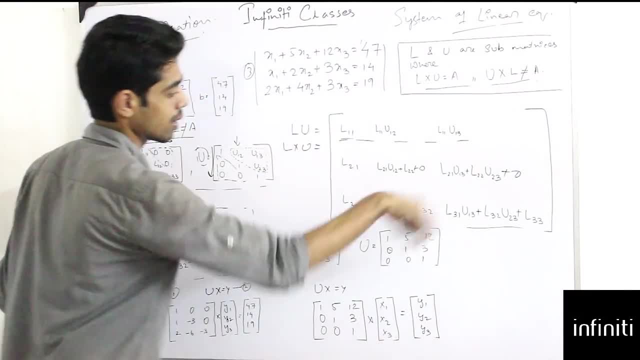 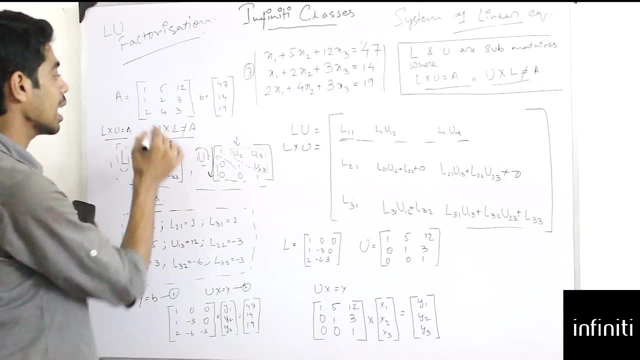 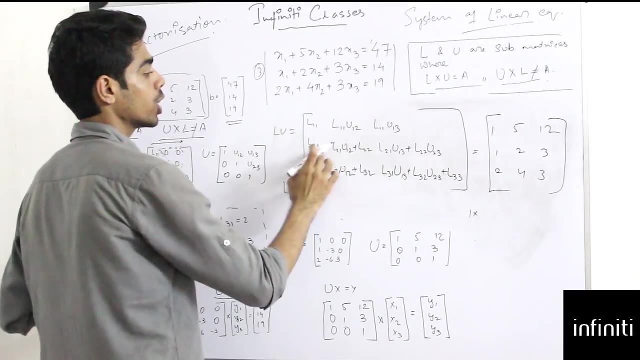 and the matrix multiplication of l cross u. is this form okay? now, as i have previously said that l cross u is equals to a. what is a? a? is this matrix okay? as we know, lu is equals to a, which means l11 equals to 1, l21 is. 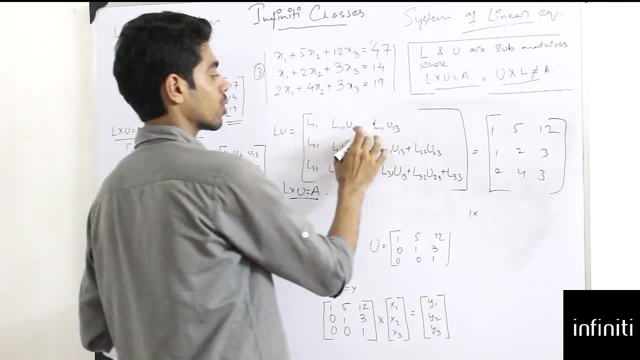 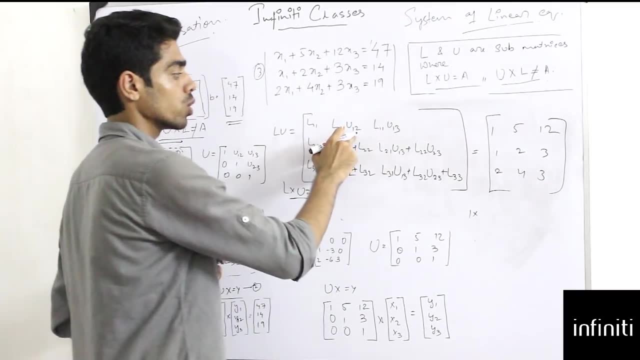 equals to 1. l31 is equals to 2. okay, now i'll calculate this one from where i'll get l12. okay, as you know, n11 is equals to 1. 1 into u12 is equals to 5, which means u12 is equals to 5. 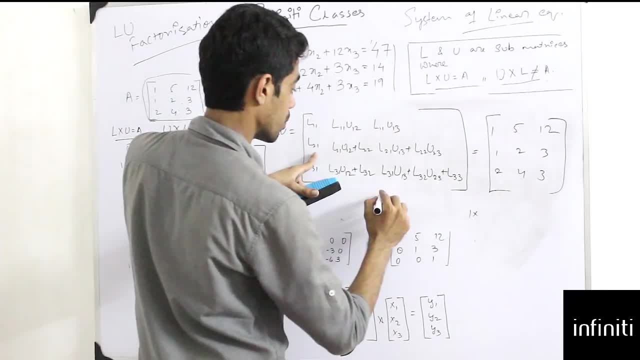 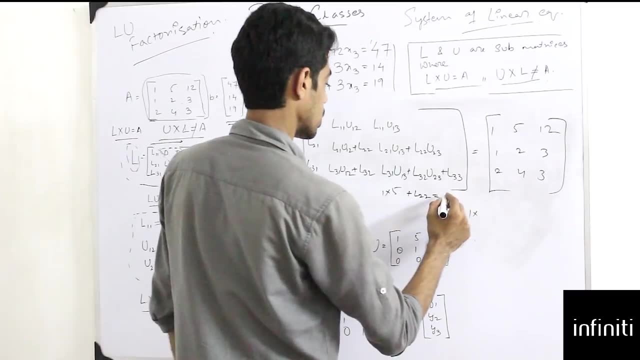 and simply we'll calculate this: l21. l21 is 1 into u12. what is u12 is 5. l22 is equals to 2. okay, 5 will be go over there. 5 will go over there. l22 is equals to minus 3. 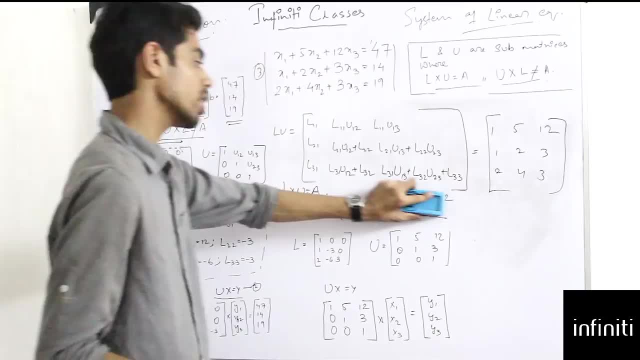 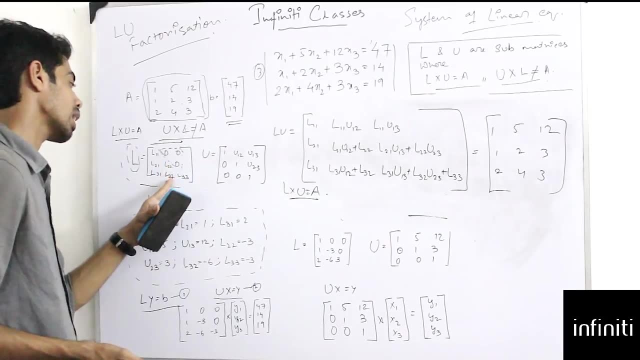 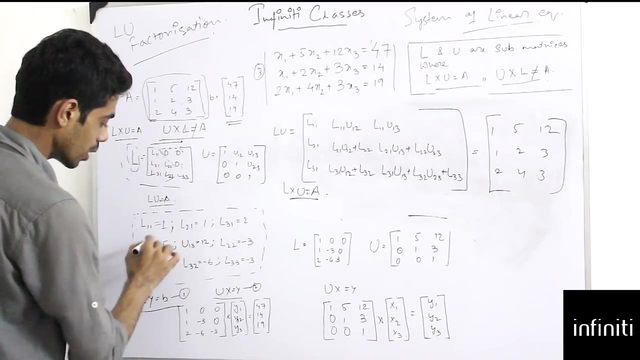 you'll get: l22 is equals to minus 3. okay. similarly, you will calculate for each and every part. means you'll get l11, l21, l22, l31, l32, l33, u12, u13, u23, okay. 1, 2, 3, 4, 5, 6, 7, 8, 9, 9 values: 1, 2, 3, 4, 5, 6, 7, 8, 9, okay. 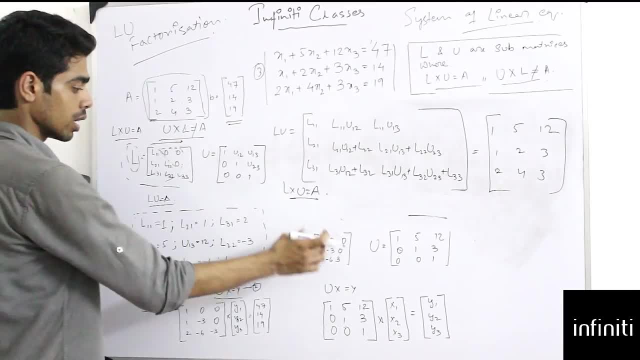 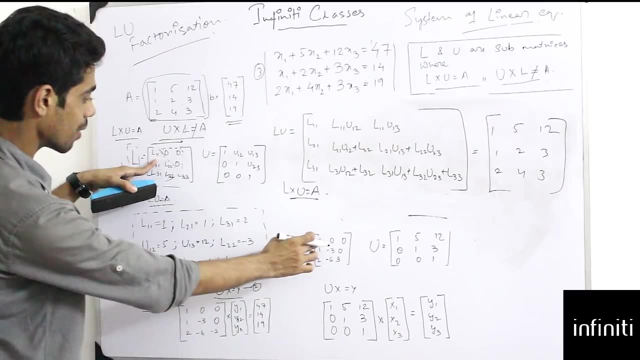 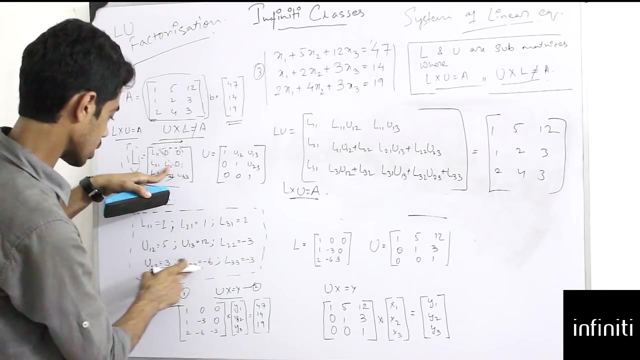 9 values. now i'll put these values and make l and u, okay. similarly, l11 is equals to 1. i have put over, i have just kept the value over there. l21, l21 is 1, 1. l22, l22 is uh, minus 3, minus 3 and. 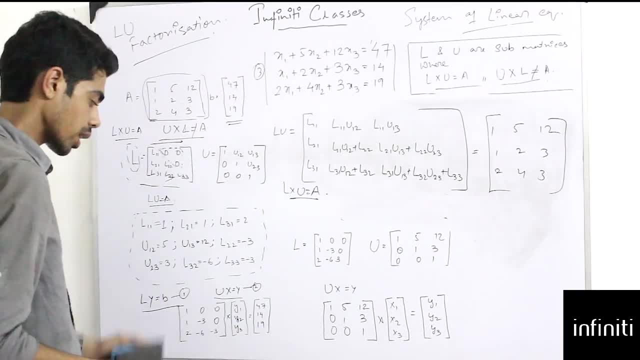 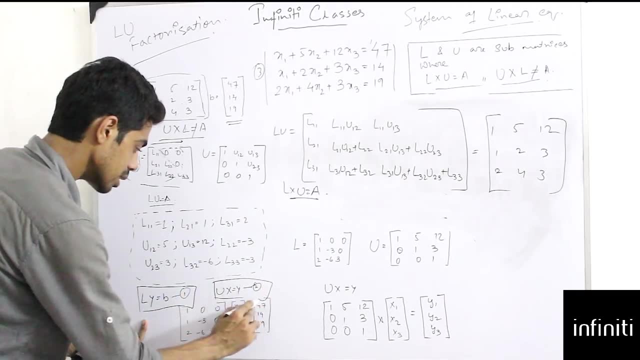 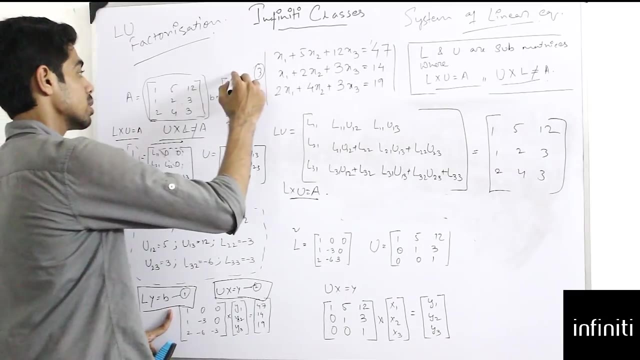 similarly, i have constructed uh, l and u from it. okay, now i have to memorize two formulas. which is ly is equal to b and ux is equal to y? okay, what is l? l is this. what is uh b? b is this. and from here we will calculate. 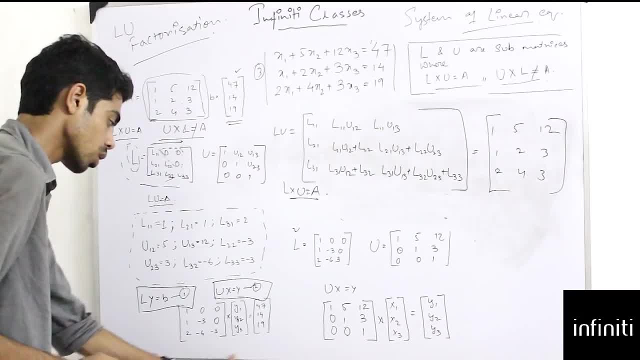 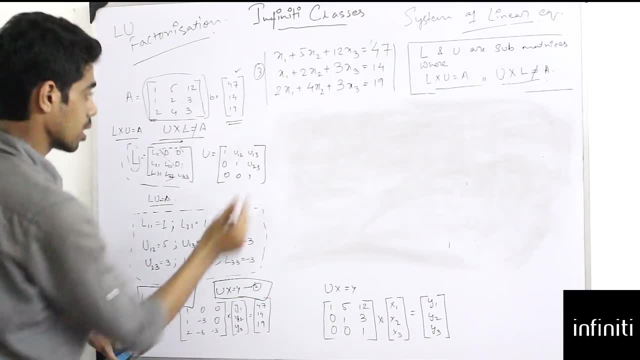 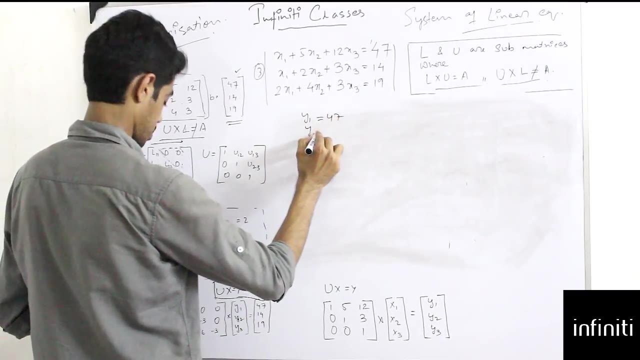 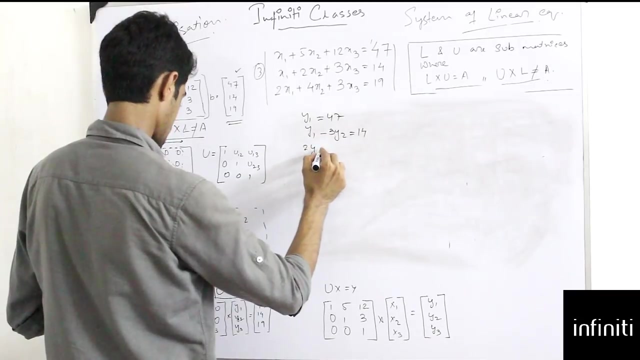 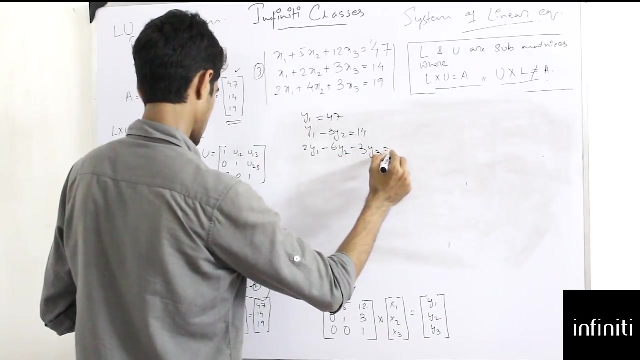 l, we will calculate y. okay, so this is my equation. now i'll calculate y from here. so what is this equation? this equation will be: y1 is equals to 47, y1 minus 3y2 is equals to 14, and 2y1 minus 6y2 minus 3y3 is equals to 19. okay, from here you'll get y1 equals. 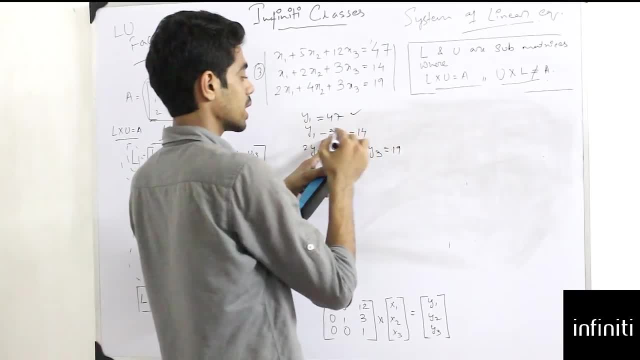 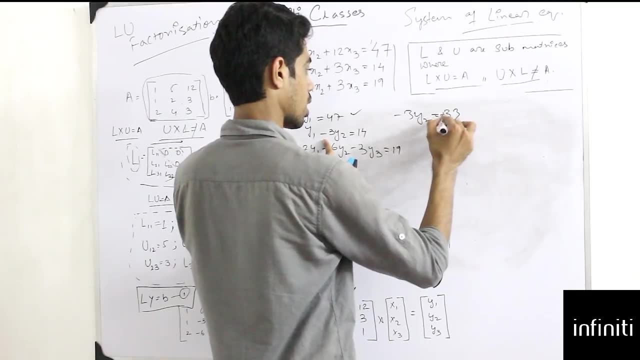 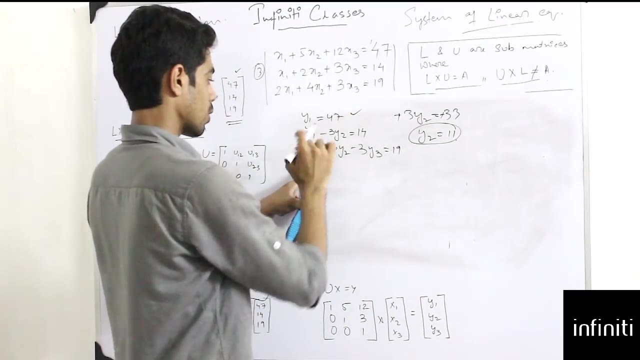 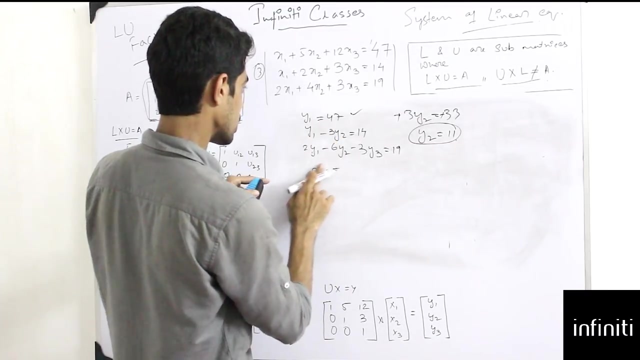 to 47. i'll put 47 over here. 47 will go over there. so minus 3y2 is equals to uh 33, right, yeah, 33 and y2 is equals to 11. okay, now i'll put y2 and y1 over here, which will i get uh 22 minus 6 in 2y1. 47 into 2 is 84 minus 6 times. 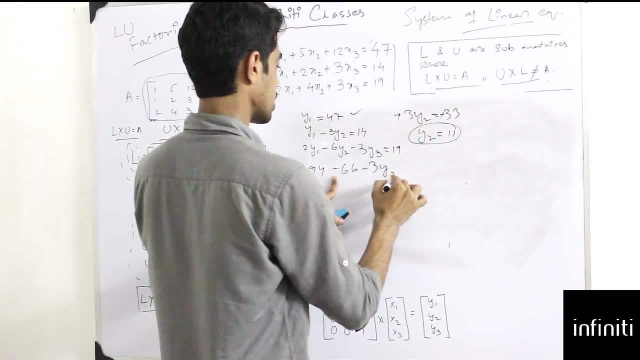 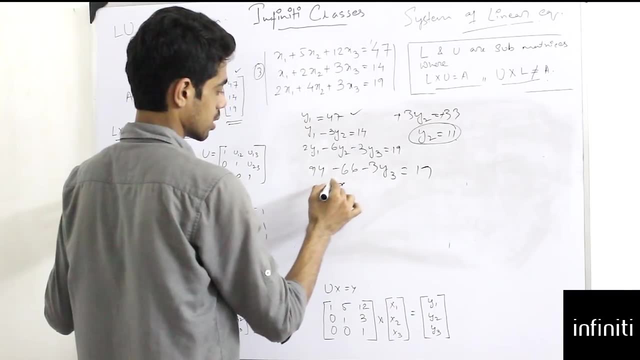 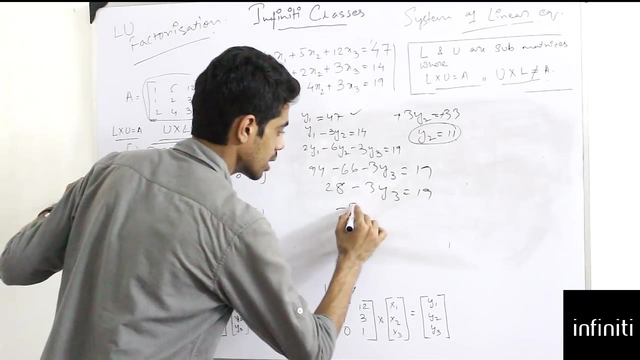 of y2, which is 66 minus 3y3, is equals to 90.. now if i subtract this from this, i'll get uh 8, and then 28 minus 3y3 is equals to 19.. 28 will go over there minus 3y3 is equals to. 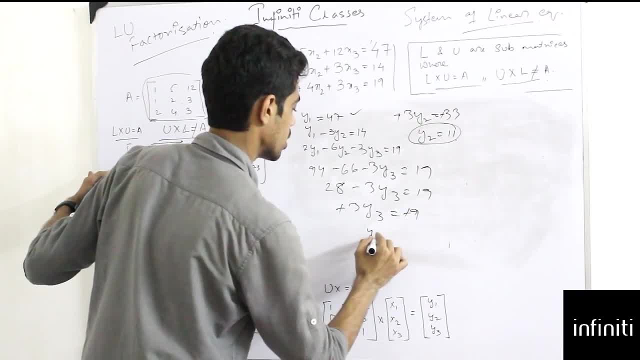 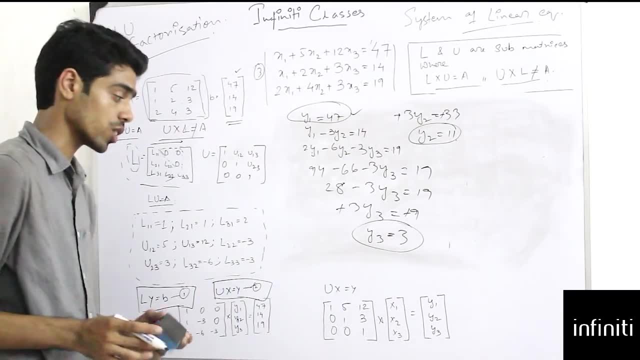 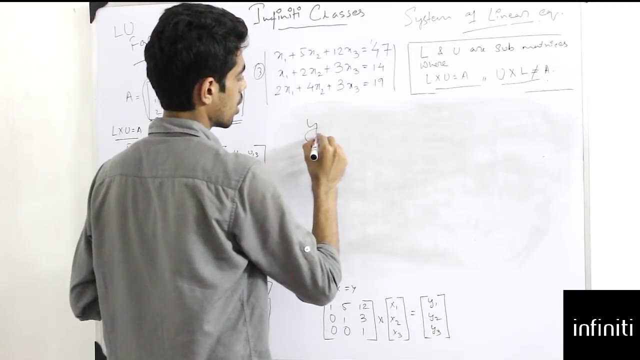 9 minus 9 and y3 is equals to 3. okay, so i have: y1 is equals to 47, y2 equals to 11 and y3 is equals to 3. okay, i put all these values over here. so what will be my y? my y will be, which is a combination? 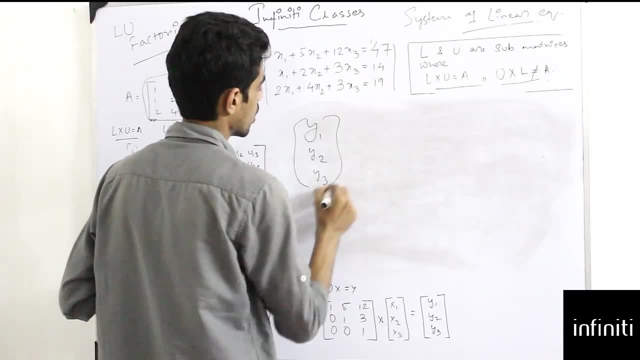 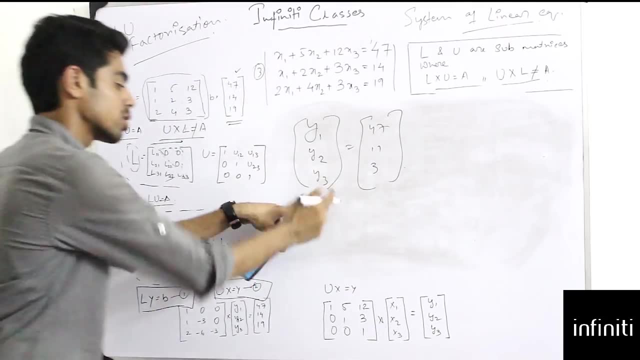 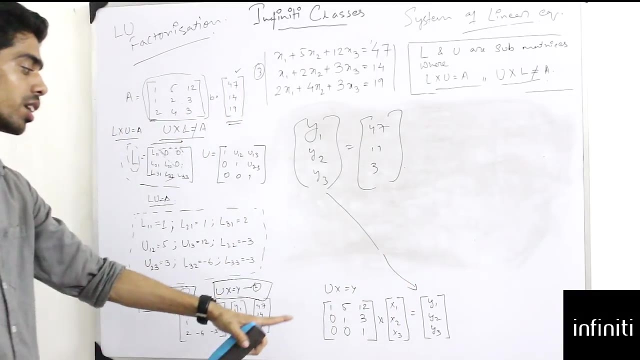 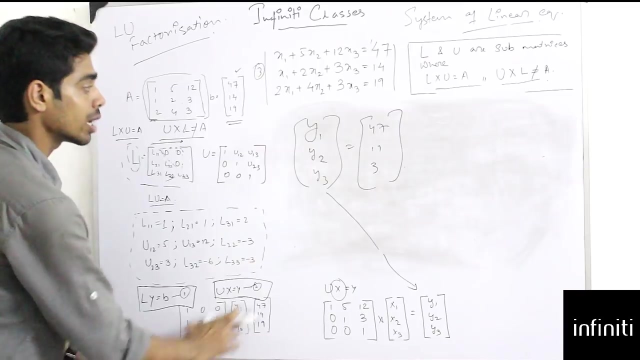 of y1, y2 and y3 will be 47, 11 and 3. okay, now i'll put this y over here. okay, i'll put my y over there to get the value of x, which is my final answer. okay, simple, i've calculated y from here. i'll put it in this. 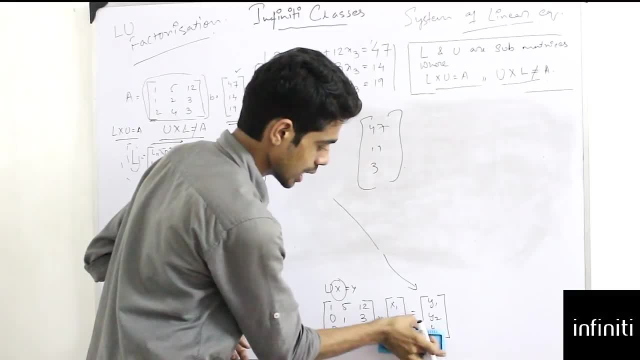 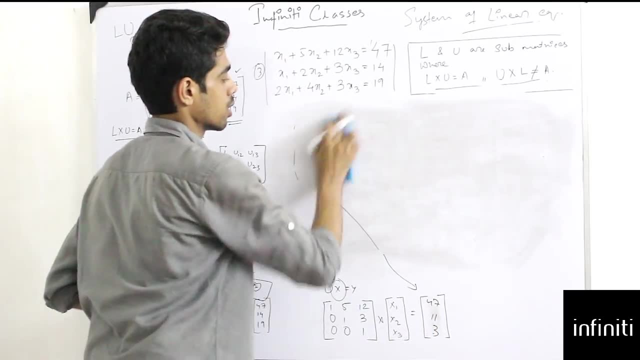 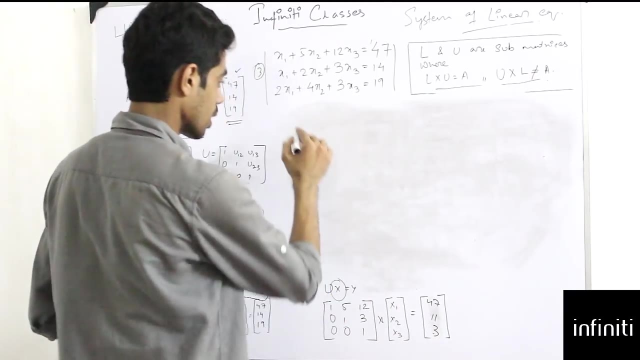 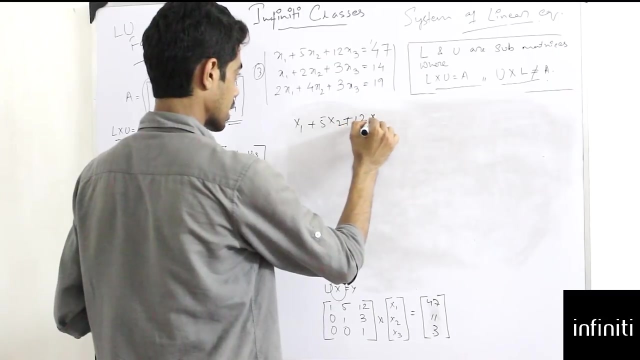 equation. okay, so what will be my equation? i'll just exchange y1, y2 and y3 with 47, 11 and 3 and now i'll calculate my ux equals to y. so what is my first value? x1 plus 5x2 plus 12 x3. 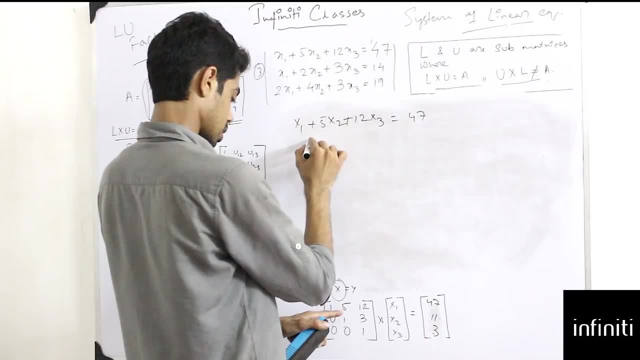 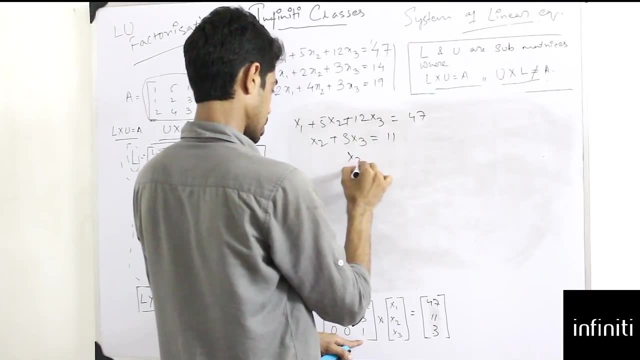 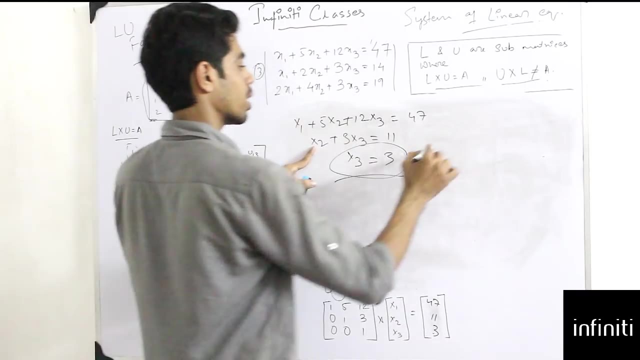 is equal to 47. x2 plus 3 of x3 is equals to 11, and then x3 is equals to 3.. okay, now from here we know x 3 is equal to 3. i'll put my this equation over here, which is x2. 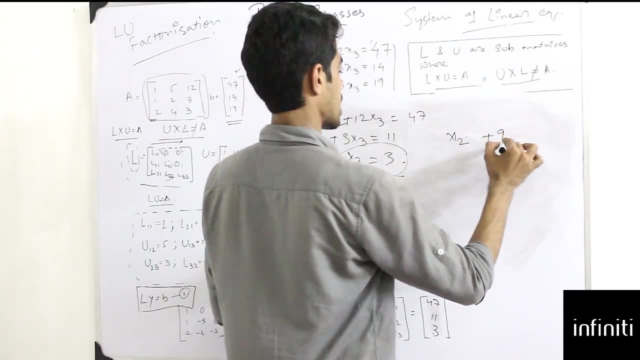 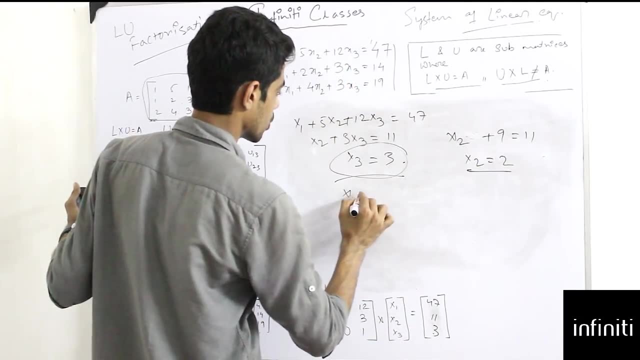 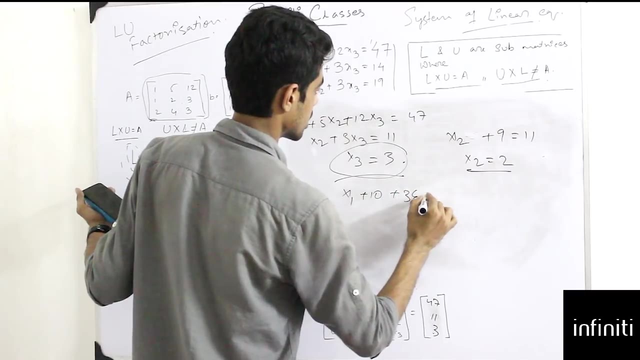 is x2 plus 3 of 3 is 9 is equal to 11 and x 2 is equal to 2, and then i'll put these equations in there here to calculate: x1 plus 5, x2 is 10 plus 12x3 is 36, express is 47 and 30, x plus 10 is 46, x 1 is equal to 47, 4. 특히, xn iş συν engraves 4. Итак, x1 ser illustrative. 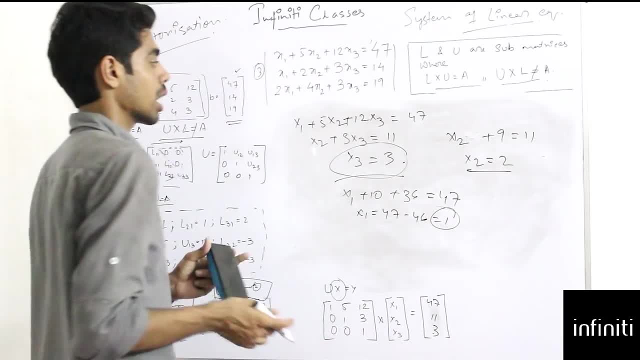 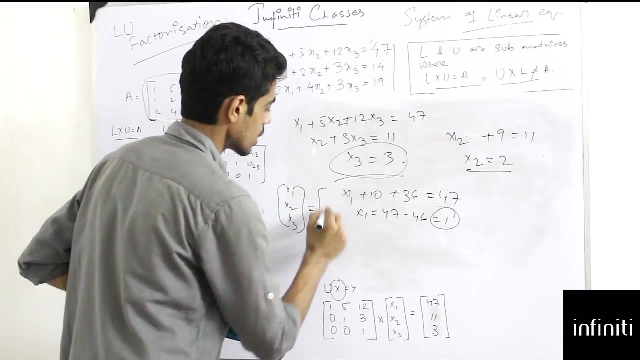 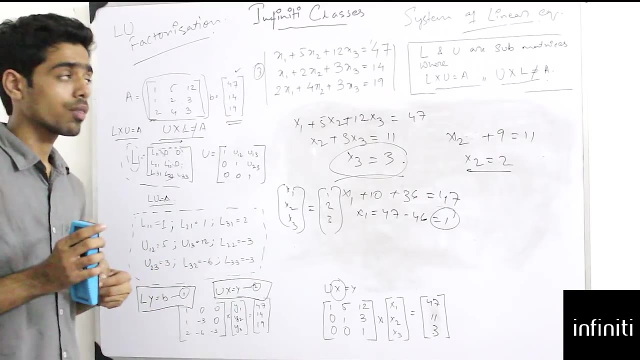 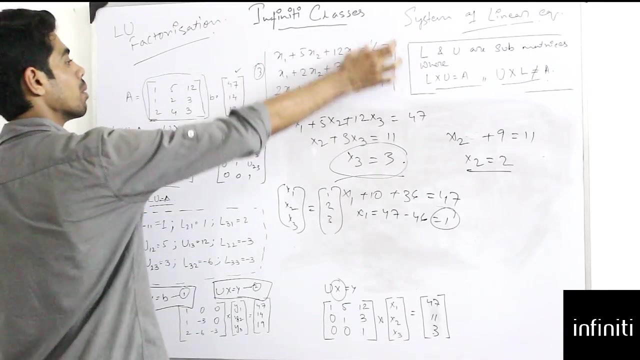 minus 46, which is equal to 1. okay, so I will get my value as x1, x2, x3 as 1, 2 and 3. okay, so this is my final answer. okay, similarly what I have done from the beginning, I have made a matrix from this equation. okay, a and b. what is my b? b is my this part and a is 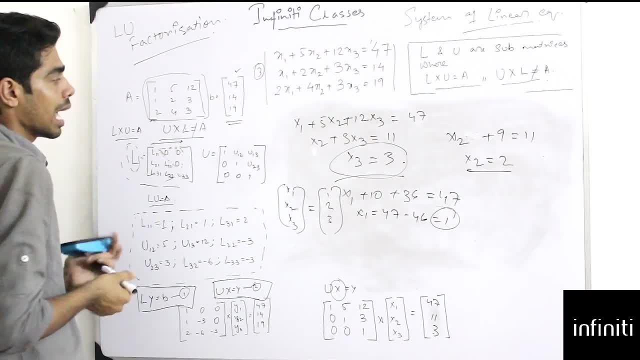 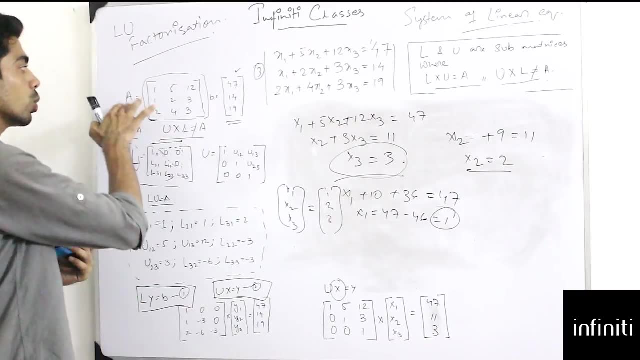 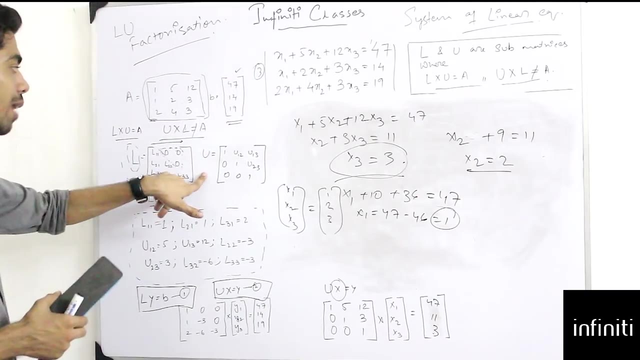 my this part. okay, now I can say that l and u are two sub matrices of this matrix. okay, so l cross u is equal to a. it doesn't mean that u cross a, u cross l is equal to a. okay, now I have calculated l and I have calculated u means I know what is l and what is u. these 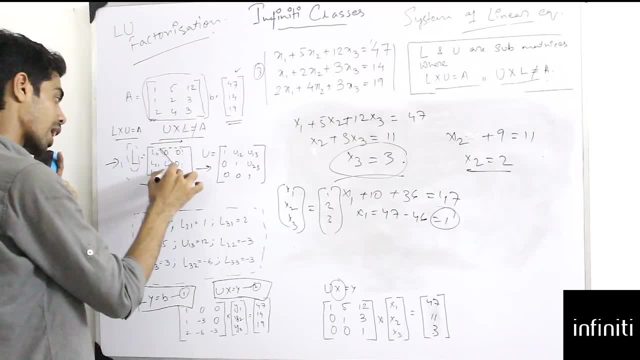 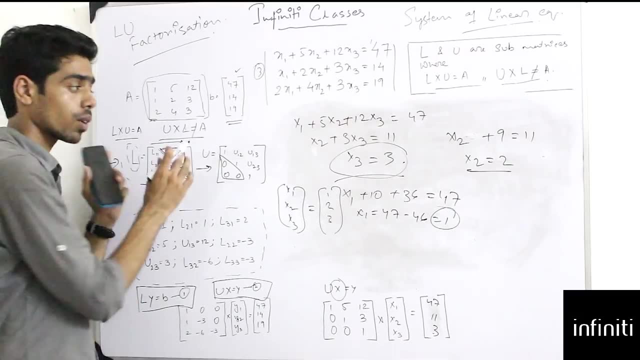 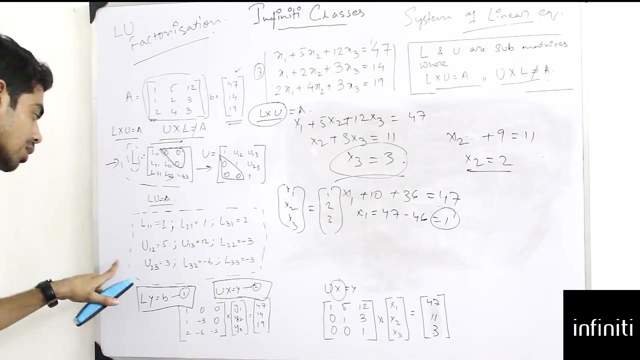 are the formulas of l and u. means: for l, the upper triangular will be 0 and for u, the lower triangle will be 0. okay, okay, now, from that I have calculated means. from that l cross u, I will find l cross u, which is equal to a. from that equation, I will calculate this equation. okay, and from here what will? 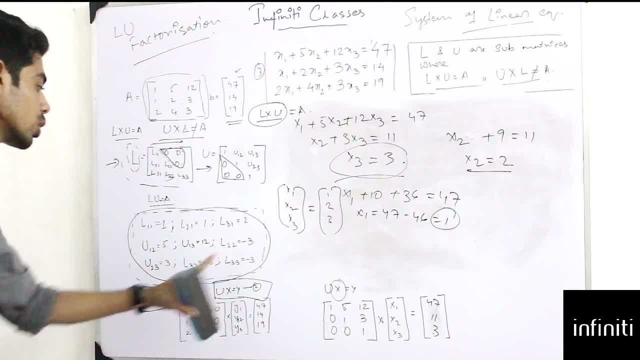 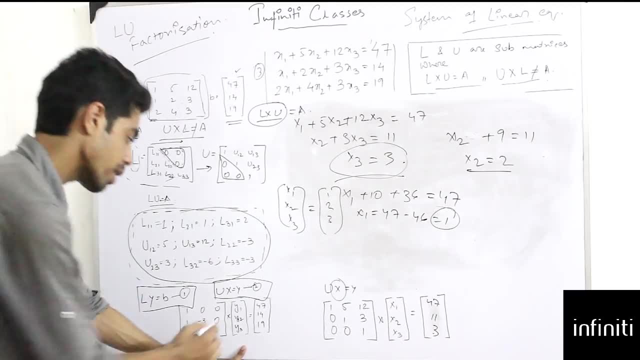 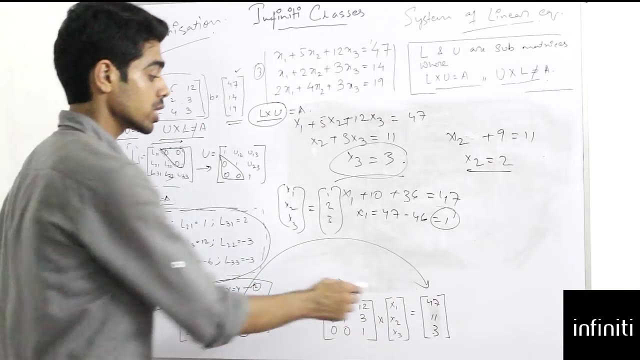 I do. I will put each and every value of l and u to their respective equations or to their respective matrices, okay, and then calculate this y1. and after calculating y1, I will put that y1 over here. okay, might x and x1 over here, right?